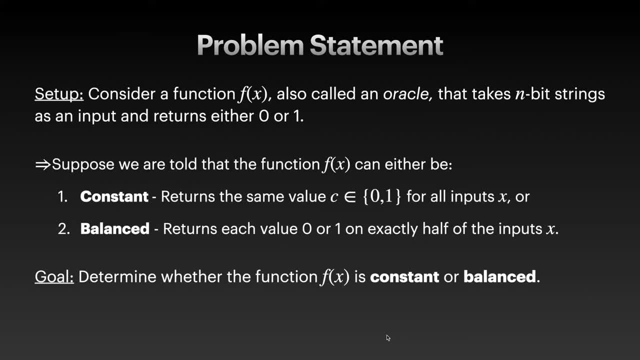 either be a constant function, meaning it's going to return the same value, either zero or one, for all inputs x, or it can be a balanced function, meaning it returns an equal number of zeros and ones for all of the inputs x. So the goal of our algorithm, 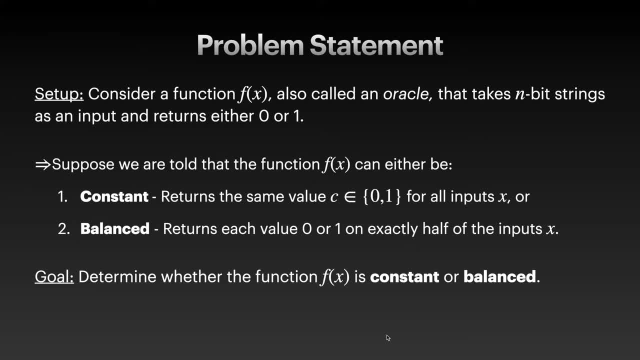 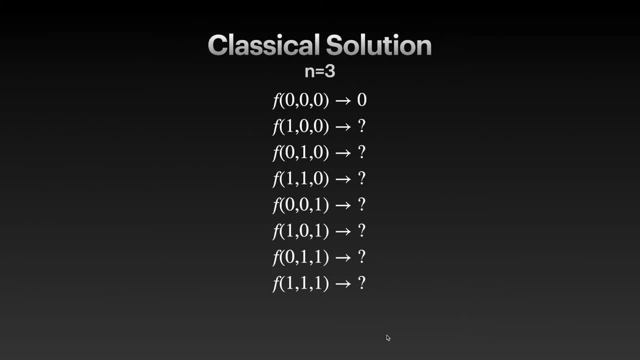 is to determine whether the function f of x is constant or balanced. So how do we do this classically? Well, let's consider an example where n is equal to three, and the only way to really do this is to test the inputs and see what values we get as output. So we test the first input. 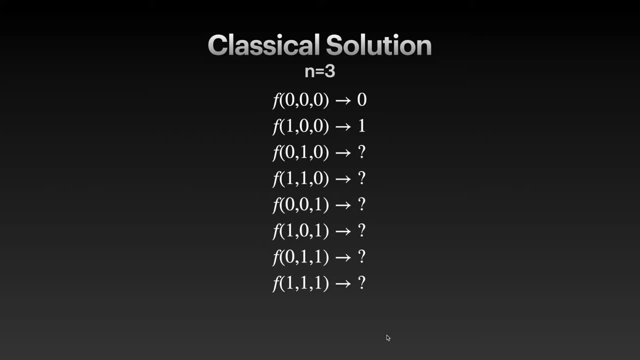 zero, zero, zero, and we get a value of zero. Now, if we test the second input and we get a value of one, we know that this function must be balanced, because the alternative would be constant, where all the outputs are the exact same. So we test the first input and we get a value of one. 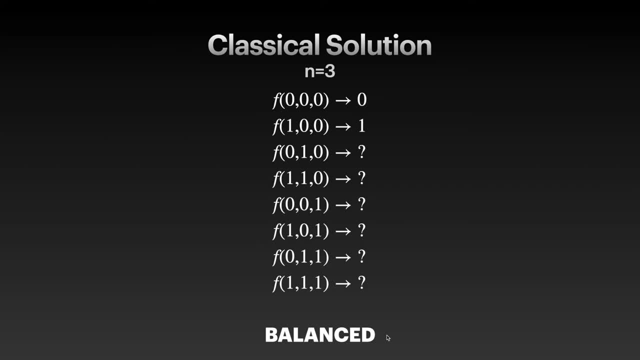 so this must be a balanced function. Now let's think about what happens when we are given all zeros in our outputs. How many of these inputs do we need to test before we know for certain that this function must be constant? Well, if there are n bits, there are two to the n total inputs. 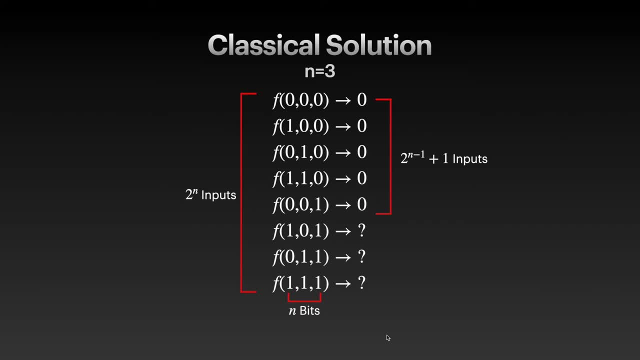 that means we have to test two to the n, minus one plus one inputs, or we have to test exactly one, more than half of the inputs, And if all of those return the exact same value, we know that this must be a constant function. 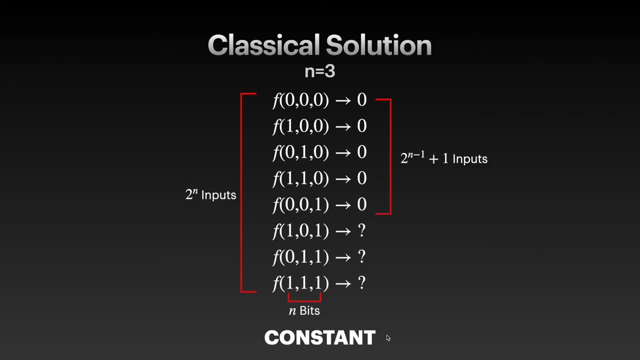 Now this is great, but two to the n minus one plus one inputs or testing. that many times can be very expensive when n is equal to a large number like a hundred. So the quantum algorithm, the Deutz-Joseph algorithm, can actually accomplish the same exact task in one iteration. 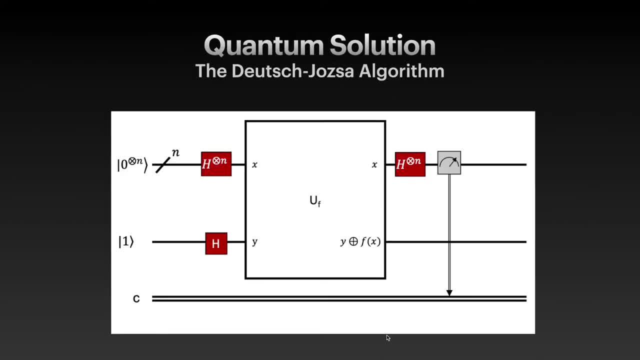 doing one calculation. So let's talk about how that works. We initialize n qubits. This top line is representative of n qubits initialized to our initial state. In this example we'll say: it's all zeros. So we initialize n qubits to zero and then we initialize. 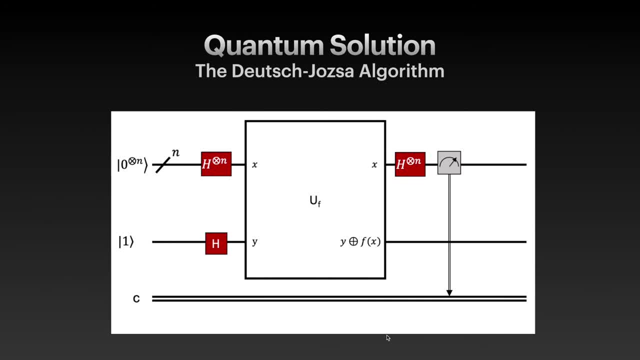 one qubit to one. Now we apply a Hadamard gate to all of our qubits, which creates an equal superposition of all states in the computational basis, and then we apply the oracle. This is this box u of f. 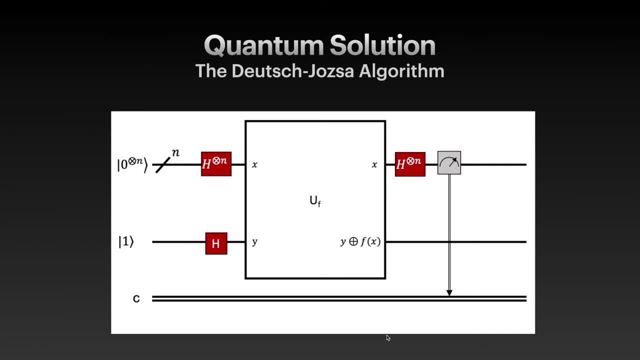 So when we apply the oracle, if it's balanced, what happens is we get this phase kickback that adds a negative phase to exactly half of the quantum states. So then, when we reapply the Hadamard gate to our zero input qubits, what we will get is a. 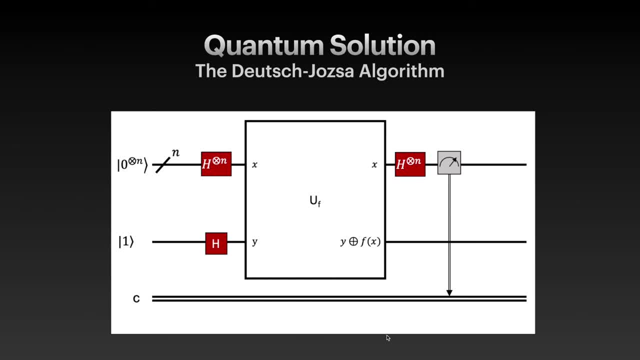 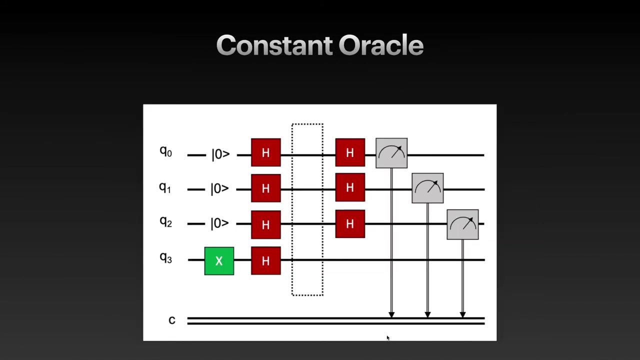 quantum state that is exactly orthogonal to our initial input state, That is, if it's a balanced function. If it's a constant function, what we will get is the exact same input state, but with a negative phase kickback. So this is the simplest form of a constant oracle. We apply our algorithm. 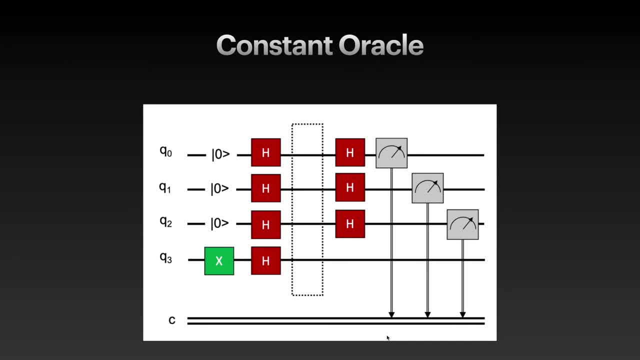 and our oracle is essentially the identity gate. It does nothing to our input. So what we should expect if we initialize our qubits to zero is that we get a constant oracle. So this is the balanced oracle. We should expect that there's a 100% chance of us measuring a zero output And 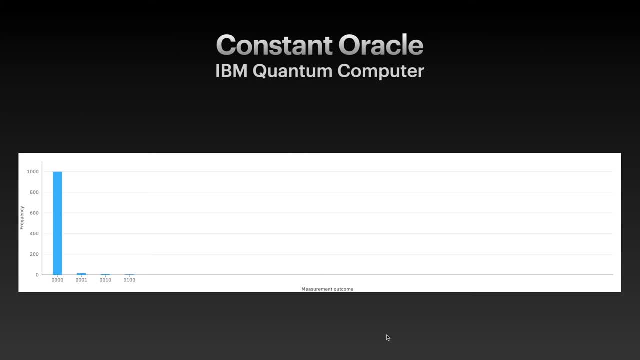 this is run on the IBM quantum computer and we see, with some small error, that the output- there's a 100% chance, there's about a 100% chance of measuring zero, as we expected. So this works for a constant oracle. Now let's look at the balanced oracle. Well, another simple example of 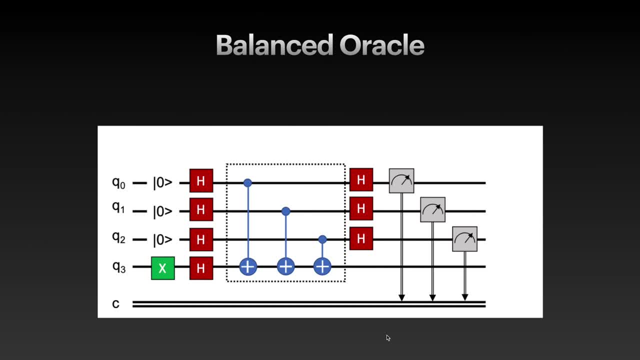 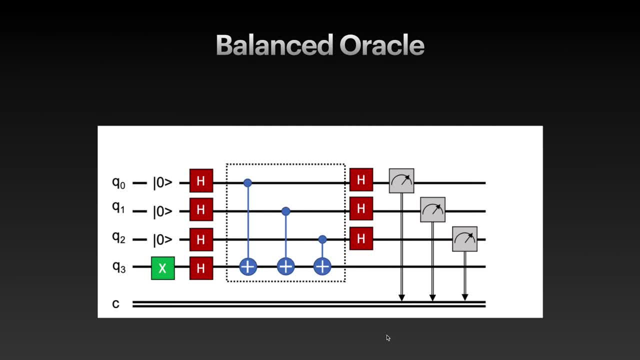 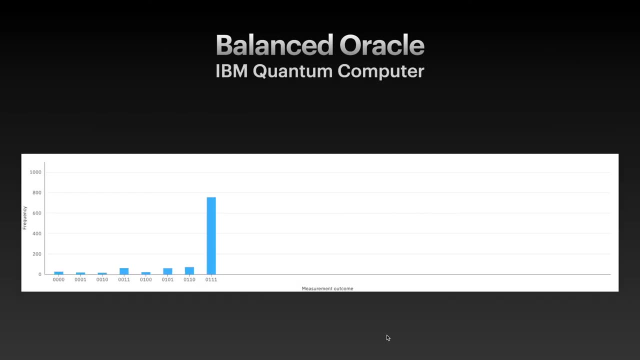 all of these zero qubits And what we should expect is, if our initial input is all zeros, that our output should be measured as all ones. There should be a 100% chance of measuring the one and there should be a 0% chance of measuring the zero string. So this again is run on IBM. 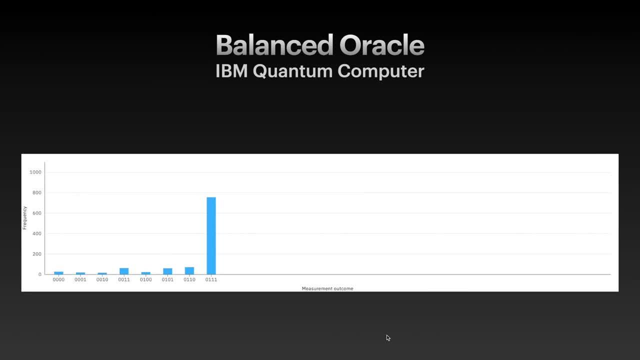 quantum computer and with some error again, we see that the probability of measuring all ones is very high, almost 100%, which means that we're not measuring all ones, So we're not measuring all ones. We're measuring all ones, So we're not measuring all ones, We're just measuring all of the. 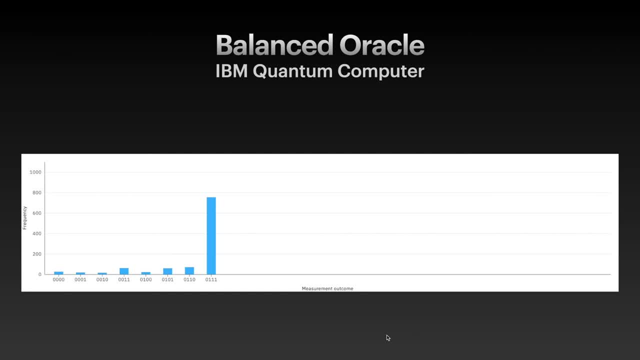 zeros. And so now we know we've done this in one iteration, which is a huge speed up compared to the two, to the n minus one plus one iterations needed for the classical solution. And that's how the Deutsch-Jozsa algorithm works. So thank you for watching the video. Make sure to like.